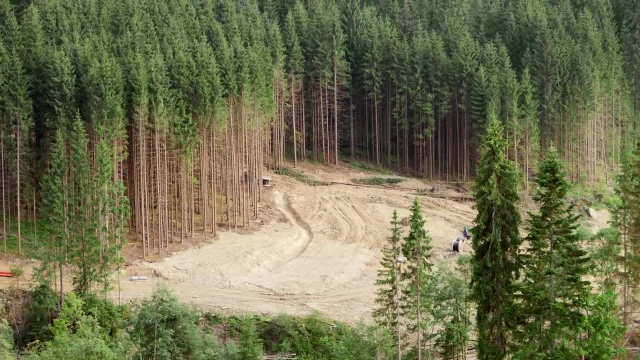 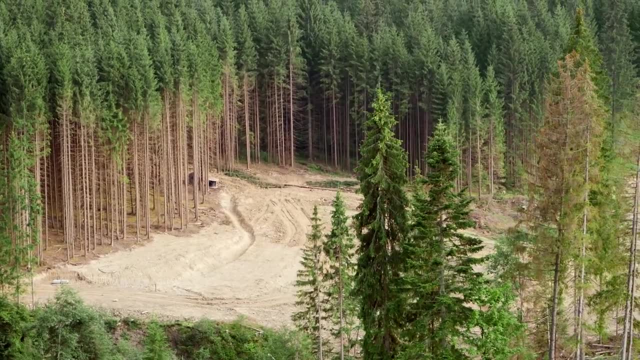 In the rainforest and other heavily wooded areas, we can see the impact of deforestation, where the forests are being cut down and sold for lumber. Many countries, especially developing countries, remove their forests and rainforests in order to generate more profit and trade with other countries. 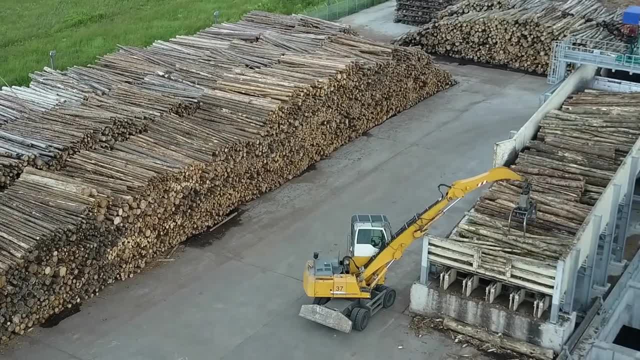 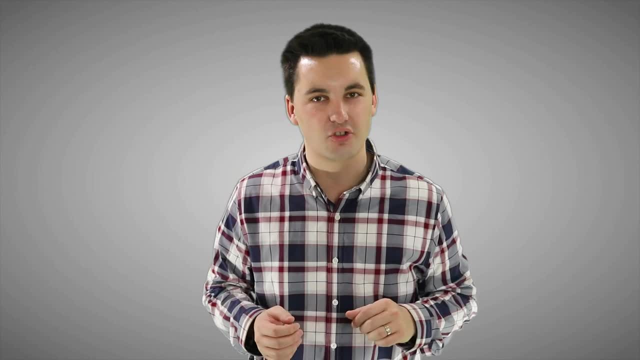 They'll also remove the forests to create farmland or make room for different settlements. If we change our scale and talk about communities that use, slash and burn agriculture, we still see the impact of deforestation. These communities often tear down parts of the rainforest or forest and then burn the fields. This puts nutrients into the soil, which allows them to get a better harvest. However, it also puts more CO2 into the atmosphere and it destroys these unique ecosystems. Other parts of the world are struggling with soil salinization, which is an excessive amount of salt. 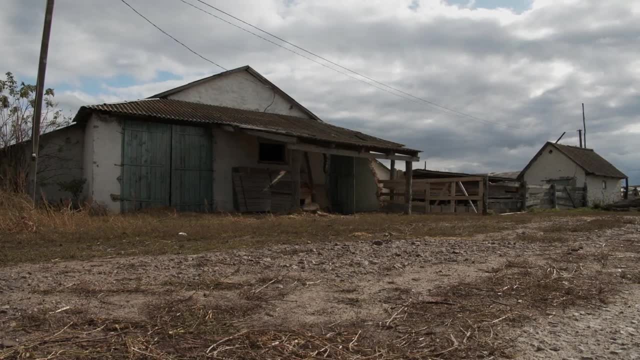 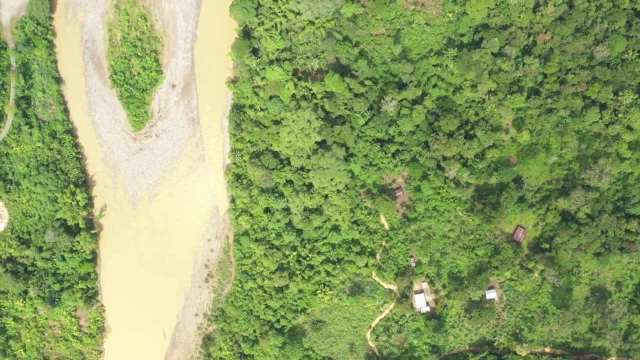 that accumulates in the soil, killing the plant roots and making it difficult for plants to grow. These areas will often see more water runoff, which will lead to soil erosion. All of this reduces the amount of arable land and it allows for more water pollution to get into the rivers, lakes and oceans. 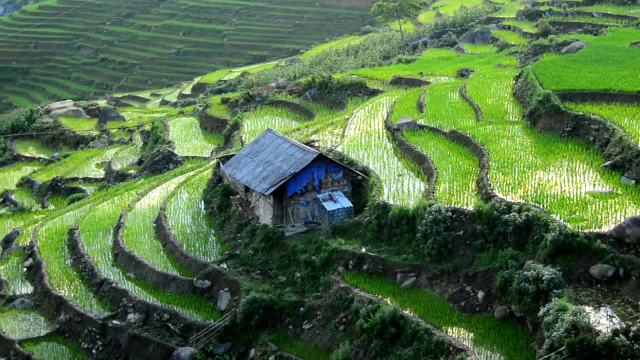 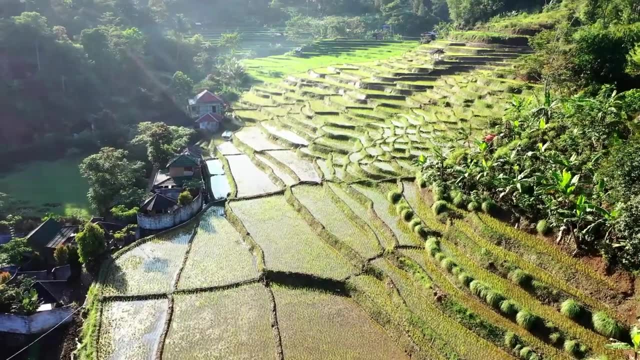 In Southeast Asia we can see terraced farming which is built into the sides of hills. This type of agriculture is like steps on the side of a mountain or hill, with rainwater running down the steps irrigating the crop. This type of agriculture is very important. 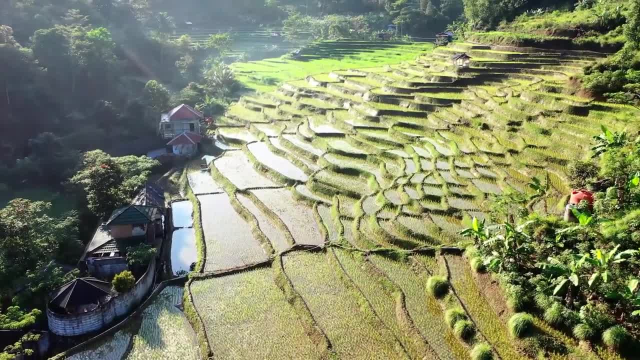 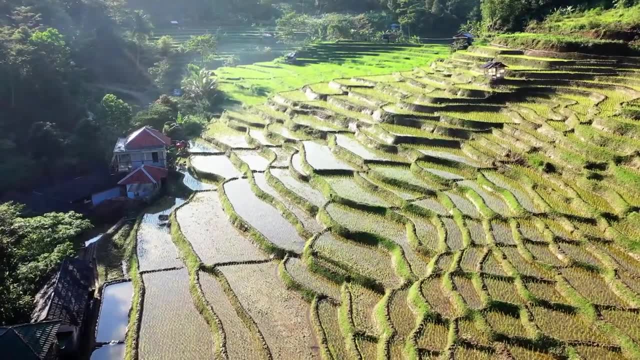 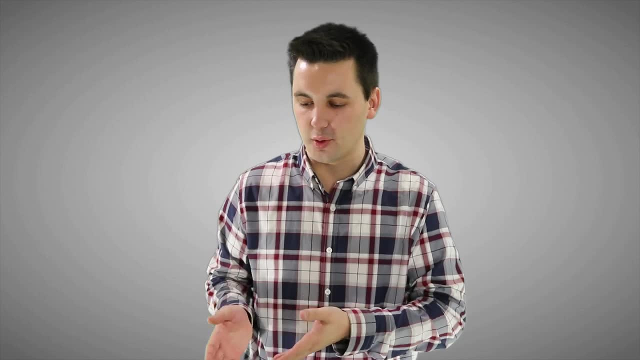 and is utilized in areas that need to maximize their arable land to feed their population, But in doing so, they also transform their natural landscape and increase the chance of mudslides. Now, throughout the world, we can see societies use irrigation. This is when we move water from one place to another. 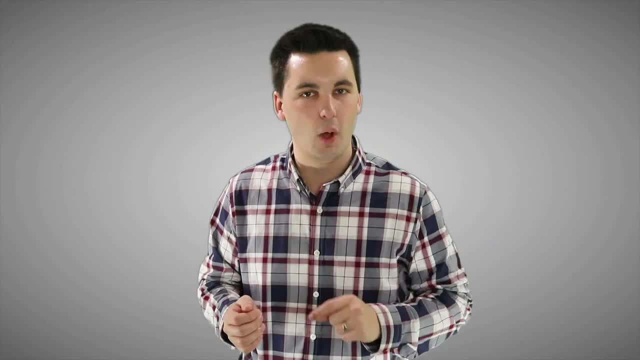 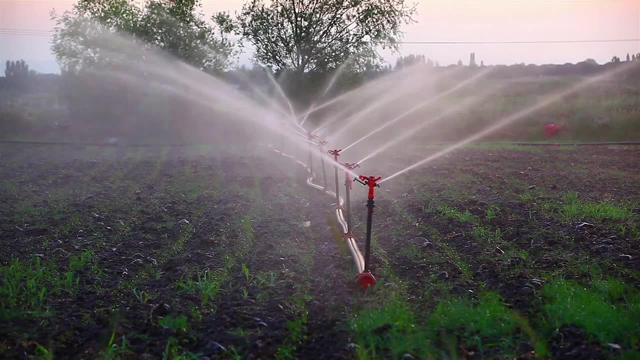 The goal here is to make sure that your crops always have access to fresh water. This allows us to plant crops in geographic areas that traditionally do not have access to water. This can be great for producing more crops, but it can also deplete fresh water sources from other areas. 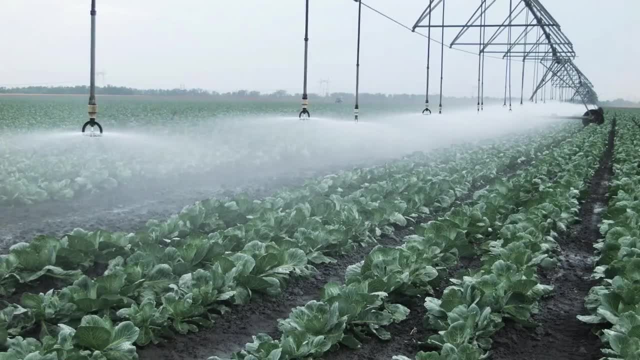 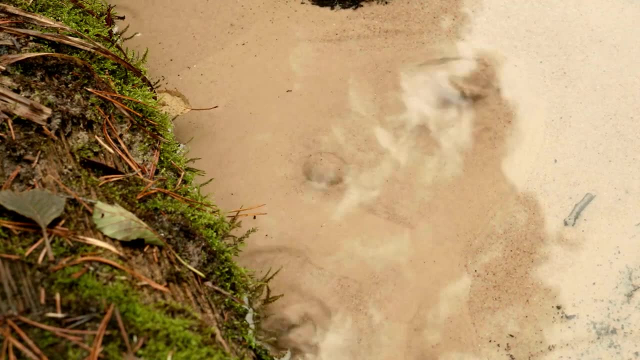 and lead to an increase in water pollution, as some of the fertilizers, pesticides and herbicides from the crops may get into the water and run off into the local water sources. On the other hand, we could look at areas that are too wet, such as the wetlands. 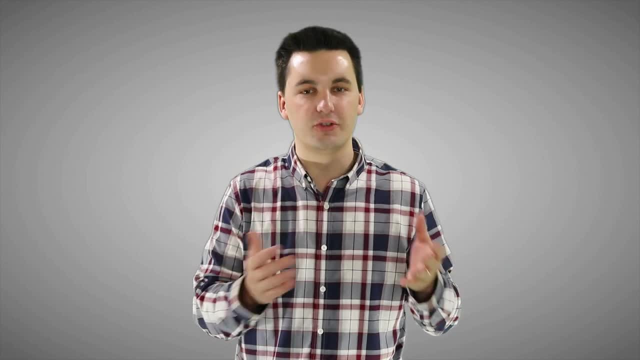 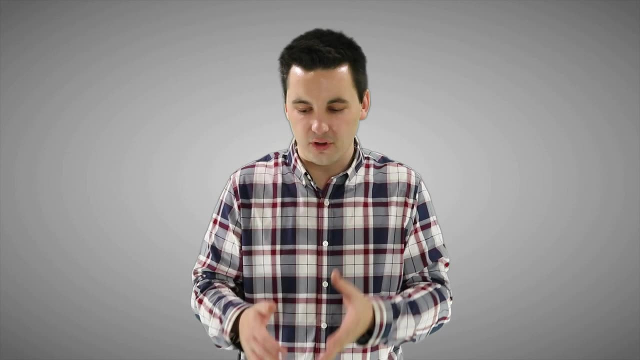 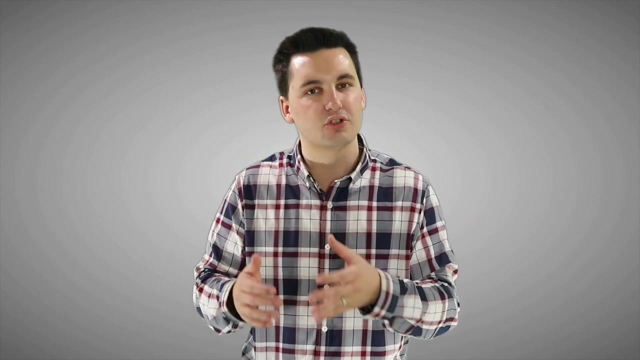 Here we can see societies draining the wetlands in order to build settlements on them and also agricultural lands. This destroys unique ecosystems and it also hurts our rivers, lakes and oceans. The wetlands act as a natural filter system. When it rains and there's water runoff, the wetlands traditionally filter that out.